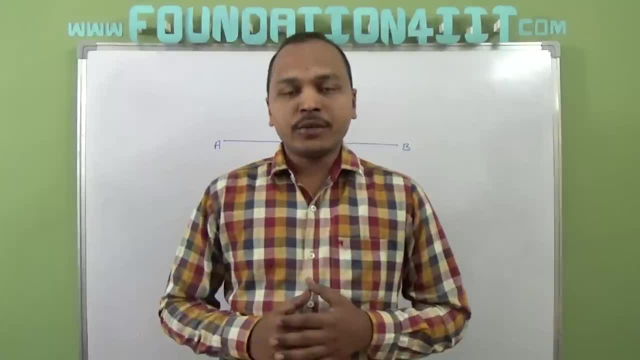 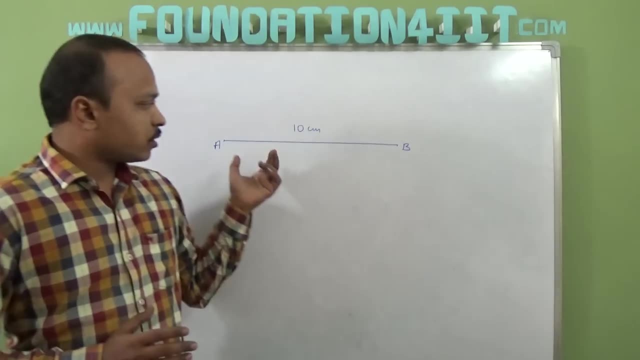 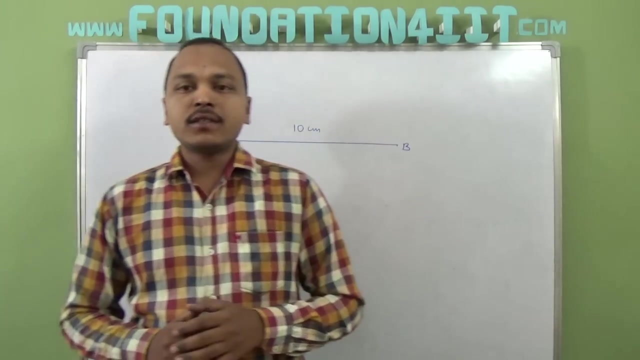 welcome to educational channel. so this video I'll explain you how to divide any line segment is given, how to divide it in given ratio. okay, in this question you observe once a line segment is given, the length of this line segment is 10 centimeters. now I need to divide this in the ratio. 2 is to 3. okay, and take number. 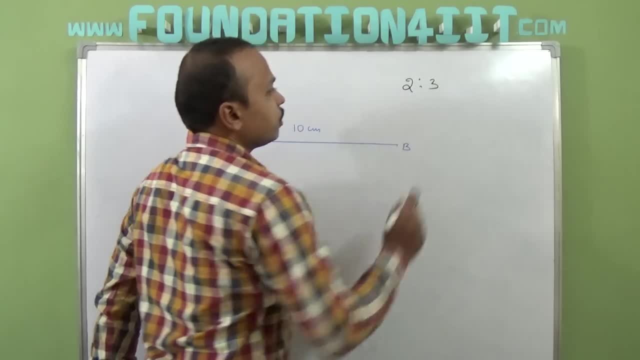 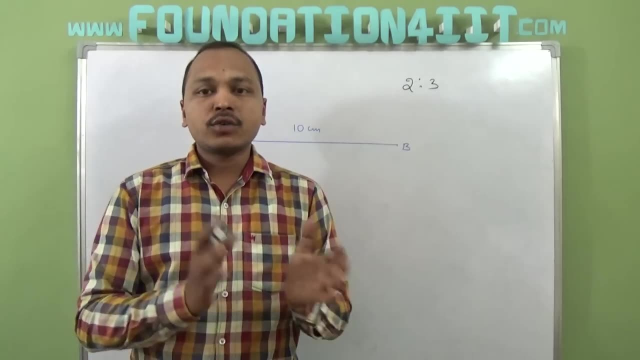 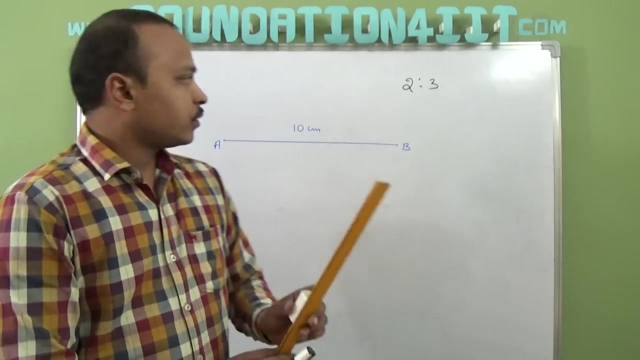 this line segment I need to divide in the ratio. 2 is to 3 means from 8 to some point, two parts, and the point to the B must be three parts, so 2 is to 3. I need to divide this in the given ratio. so the ratio is 2 is to 3. so what we should do. 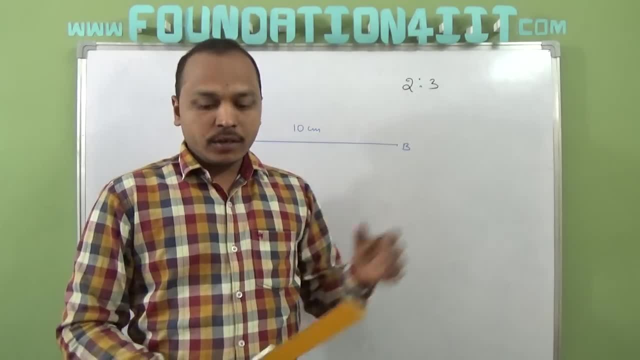 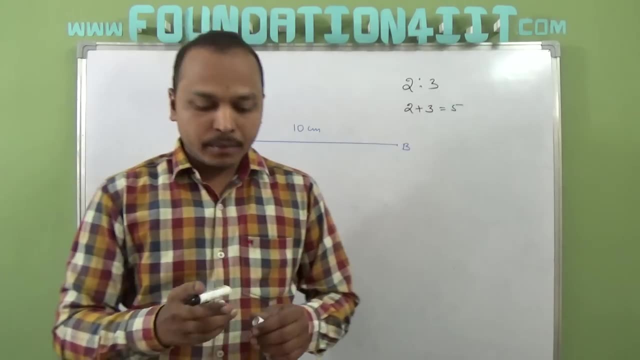 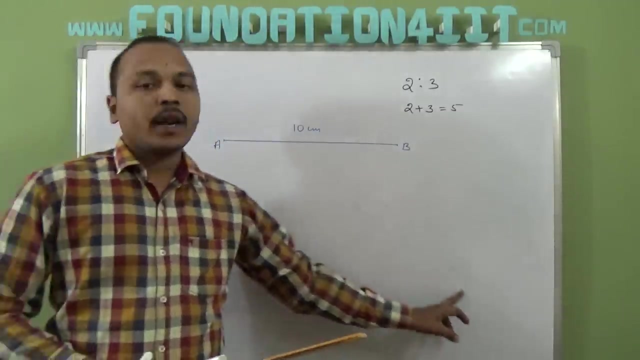 so 2 plus 3, the, whatever the ratio is given, just add the numbers first. that is, 2 plus 3 is equals to 5. so just remember that 5 number. now take this K from what point? A, which is to take a line with some reasonable angle around acute angle, not like more than 90, so any 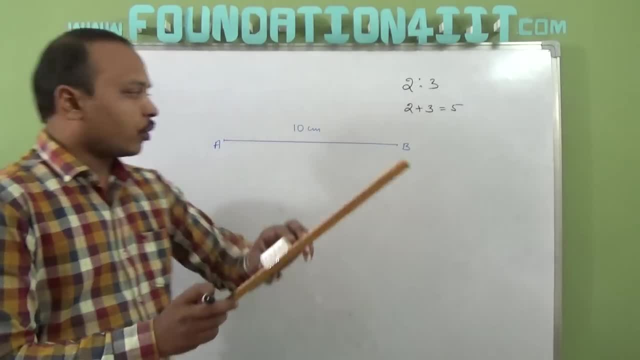 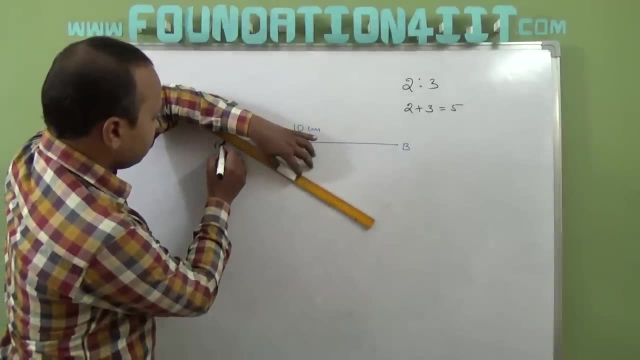 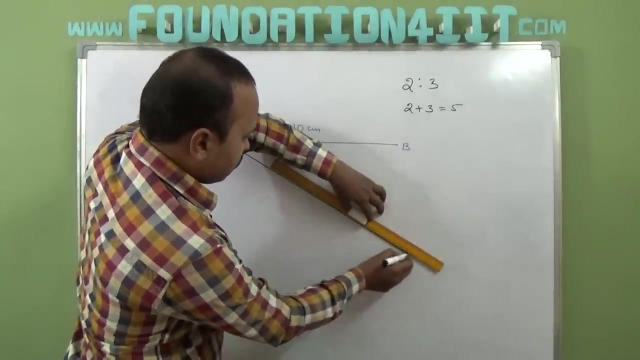 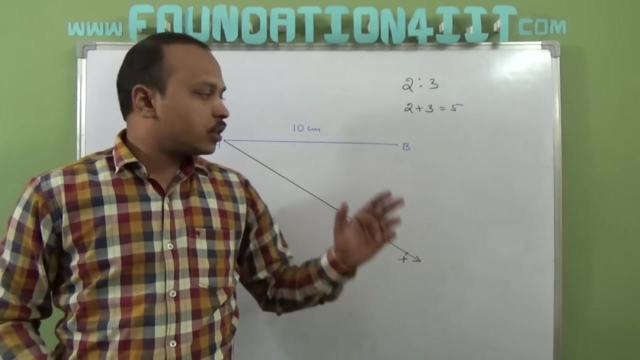 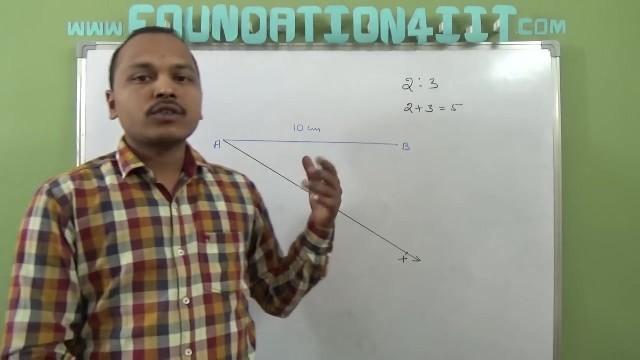 acute angle take a line towards down, so from A just take a line, so line you can draw. okay. A take some X a ray, so AX is the ray, just to draw a ray from A any angle you can take. so acute angle maybe a 60 or 70, so should. 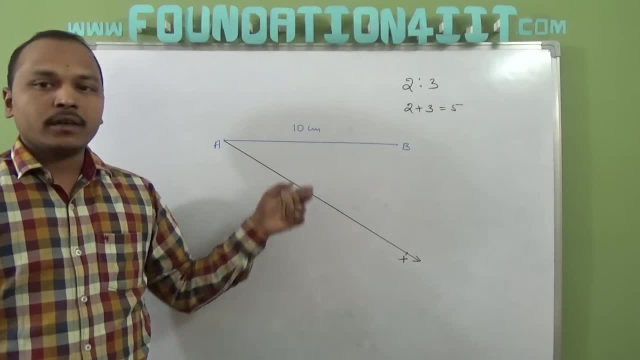 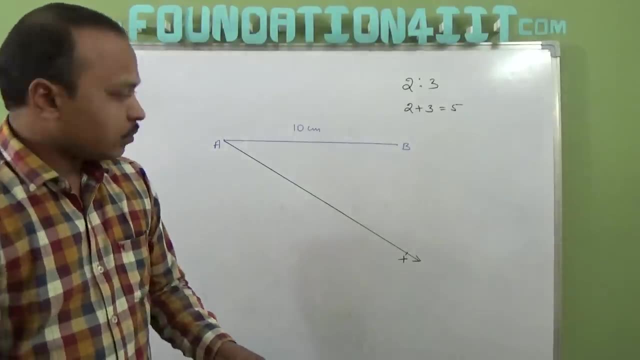 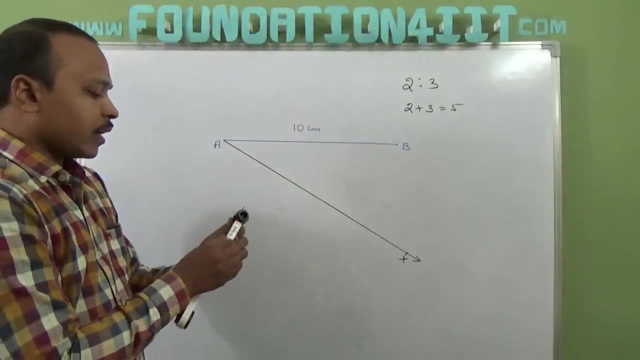 not be more than 90 and very small, some reasonable angle. you can take a line first now. if you take the numbers now we need to: 2 plus 3 is equal to 5, right? so 2 plus 3 is 5, so I should make 5 equal parts this line now using this compass. 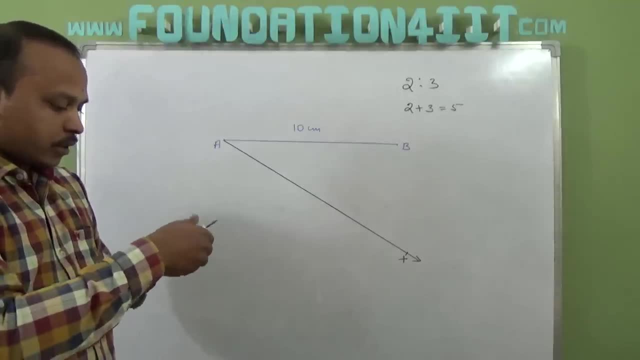 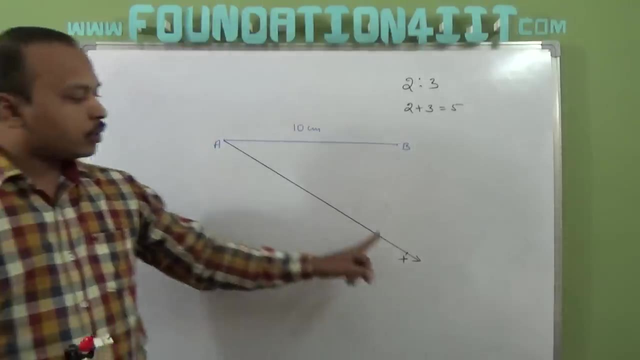 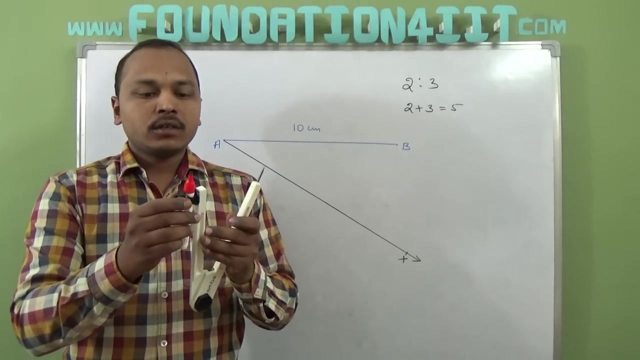 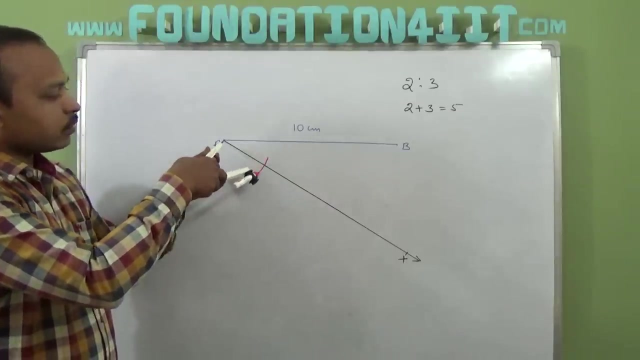 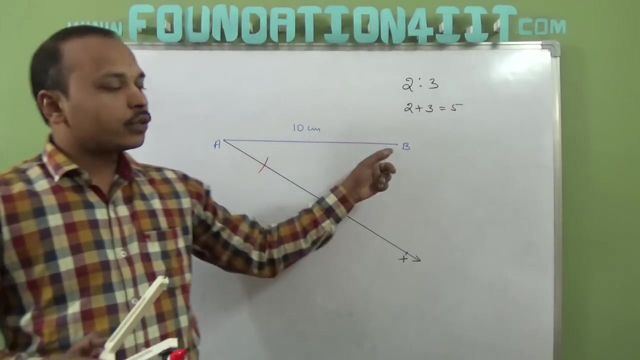 you just space. sorry, is 2 plus 3 by 2, you are making 5 equal parts, right? so this line and x is equal to one control. you do that. so the любим of the two-way mirror, yourohl ganρε, because we don't know how to cut the AB in exactly 5 parts. 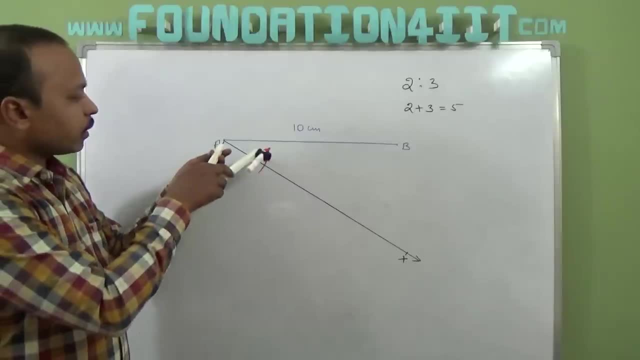 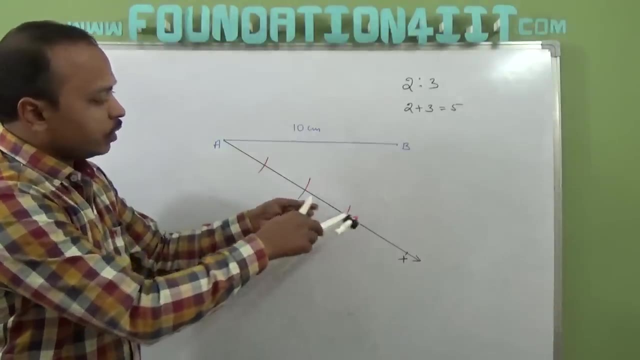 That's why you can take one more ray and that will cut into 5 equal parts. So from here to here. I did again from here, without changing this: 2,, 3,, 4, and you can extend this 5.. 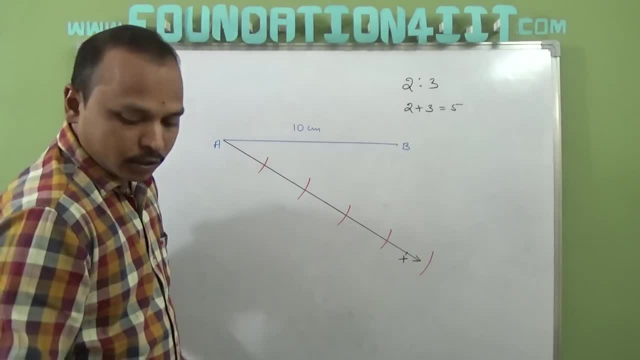 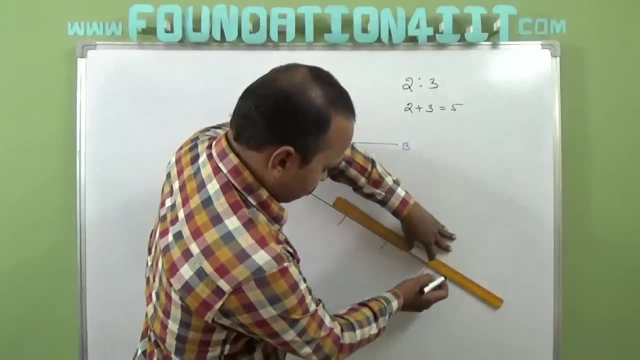 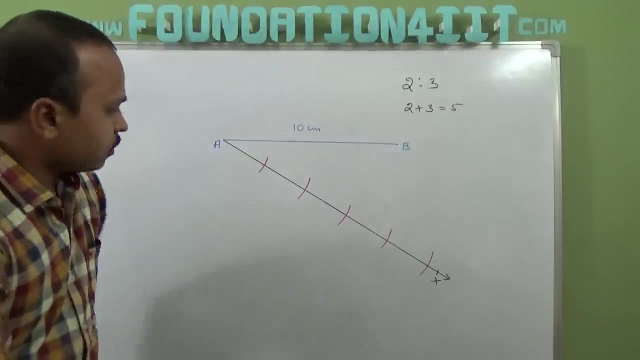 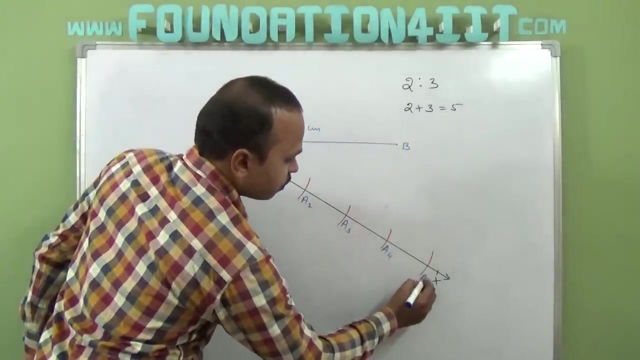 So if it's not sufficient, you can extend this also. Ray, you can extend Now the part which is cut. this is A1, A2,, A3,, A4, and A5, the parts. So AB is a 10 cm line segment. 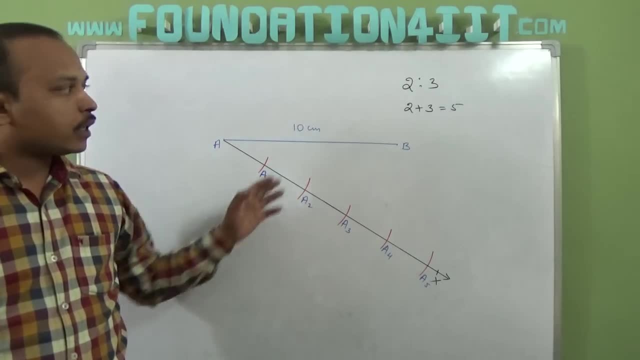 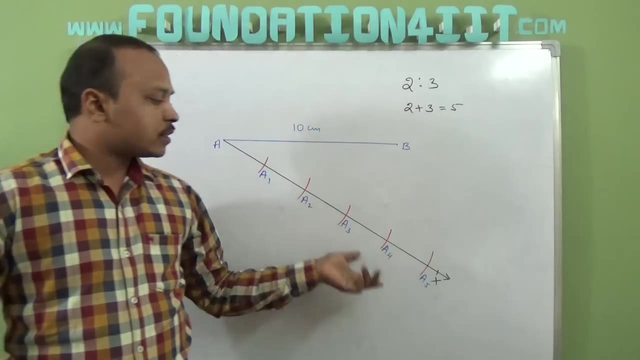 Take one ray from A towards down And that account the given ratio. If they ask, 1 is 2, 3 means 1 plus 3, 4.. So 4 equal parts. So if this number is more, this reduces small. 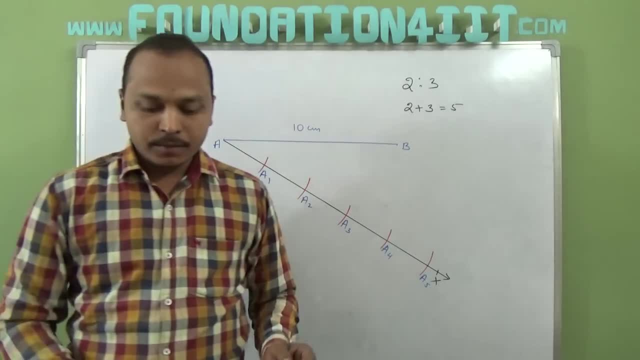 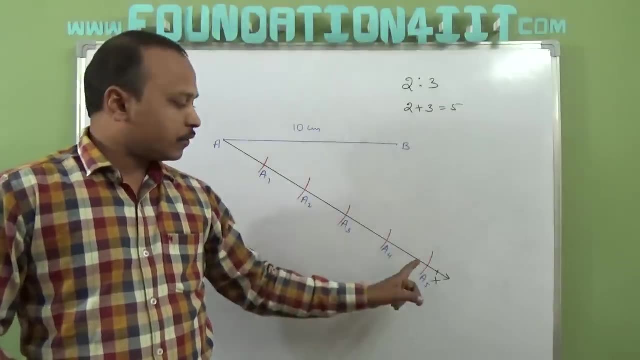 Means this radius. you can reduce and you can cut into parts. Now, A5 to B, you join Last point, because total 5 parts. So 5th point to B, you join this Scale A5 to B, you join. 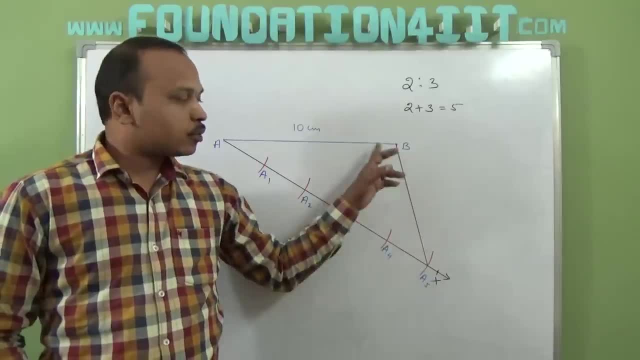 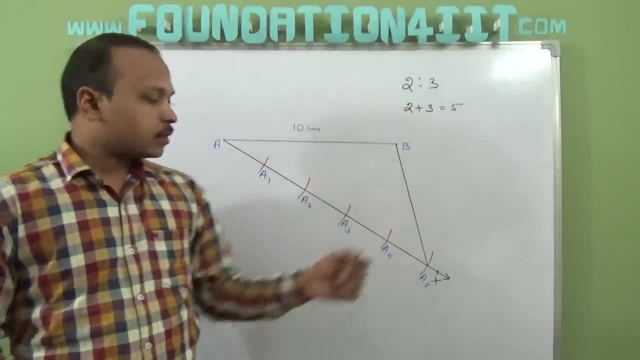 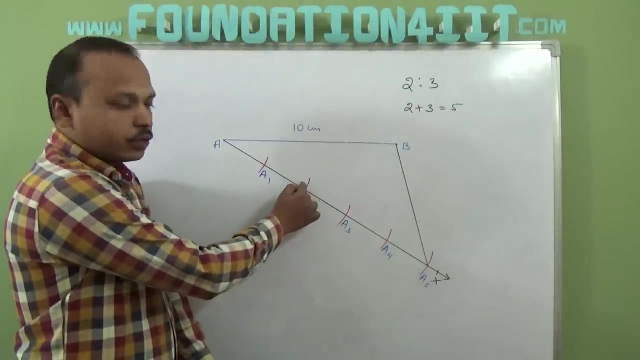 So 8 to 5, A5 to B are joining, Now 2 is to 3.. So first is 2 parts, Remaining is 3 parts. Now, from 2 you should draw 1 parallel line to this. Then from A2, I need to draw exactly parallel line like A5 to B. 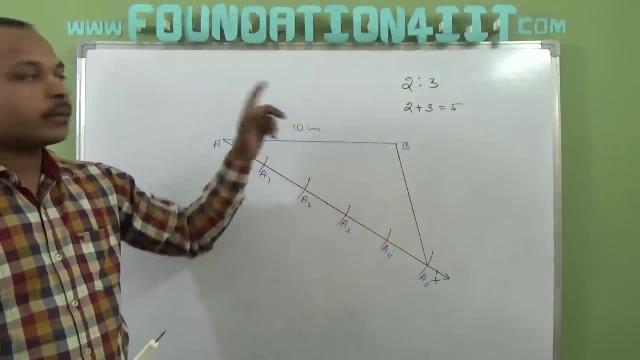 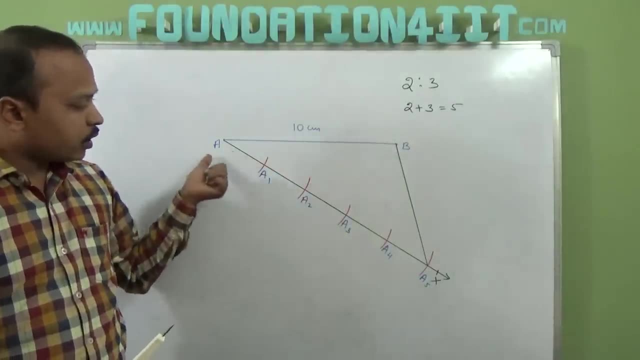 Whatever is line From A2. also, you should draw parallel line, Because we need 2 is to 3.. So this side is 2 parts, This side is 3 parts. So A1, A2, A2 is A2, A2.. 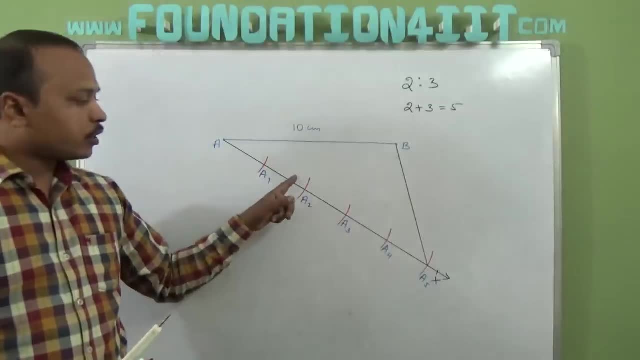 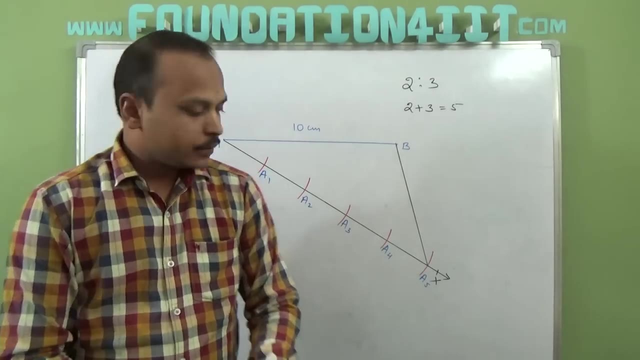 2 parts And A2 to A5 is 3 parts. That's what A2. you can draw parallel line. Exactly same line. So how to draw parallel line for the given line, you know already. Just take this from A5.. 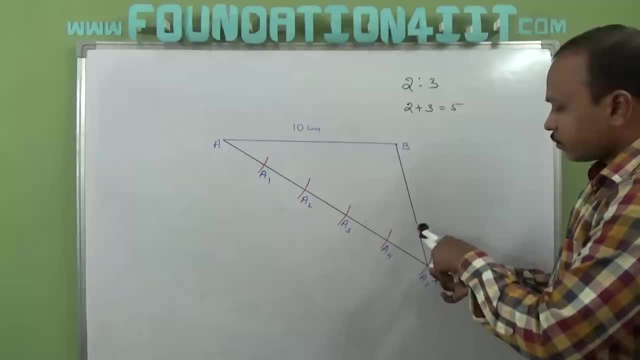 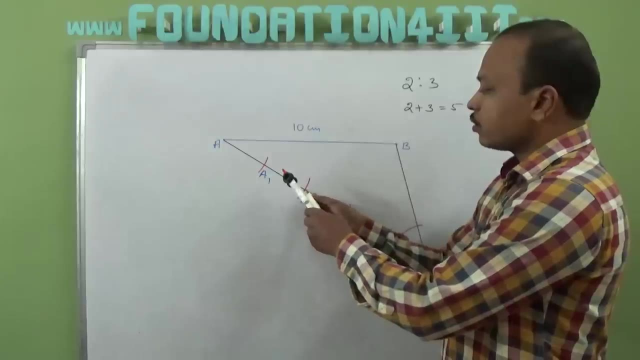 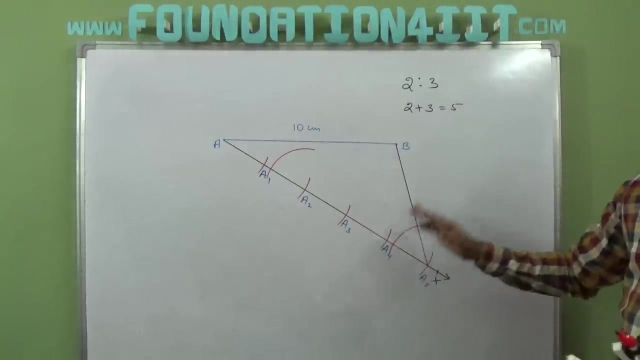 Now observe here: From A5, draw an arc Without changing this, From A2 to B, From A2, also, draw an arc. First step: From A5, draw an arc by touching this, both Without changing the radius you can draw. 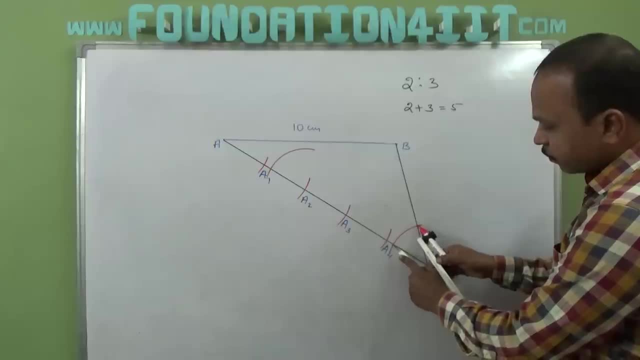 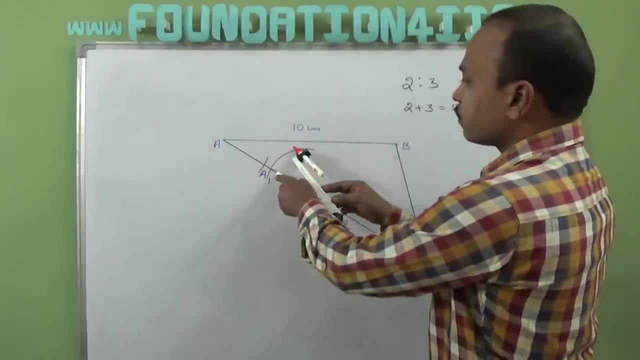 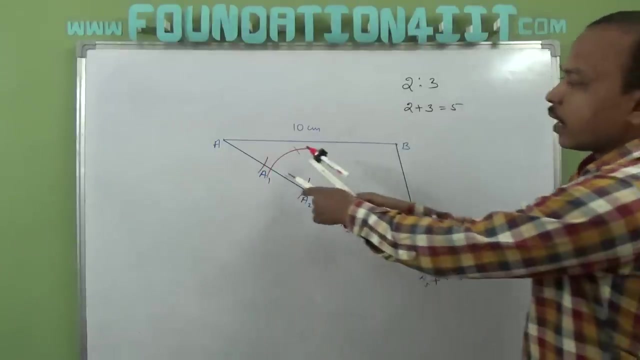 Now observe from this gap. Keep your compass like this, How much it is Now, remove From here. also, you can draw an arc. That's it Immediately. this angle should be making here same. Keep here and draw an arc from there. 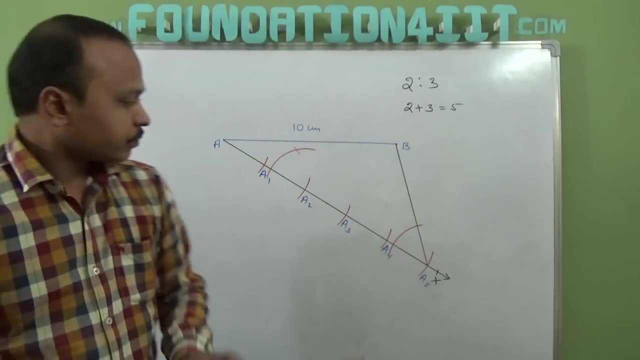 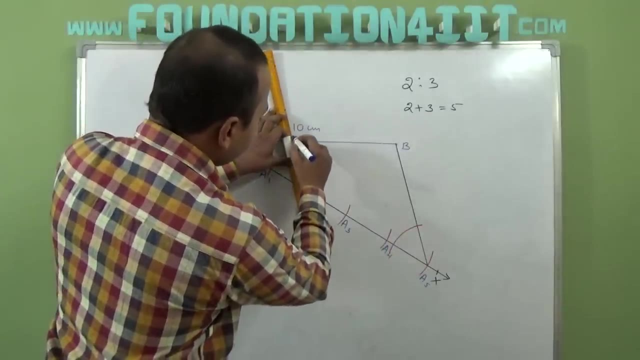 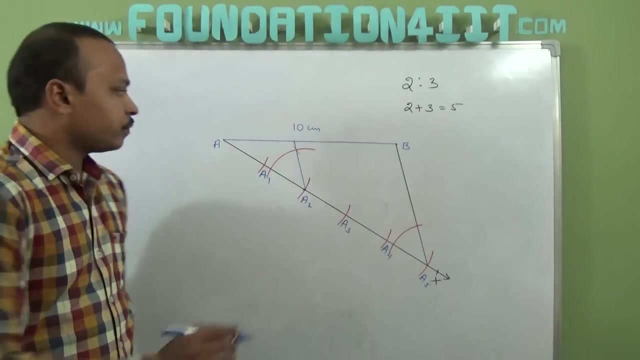 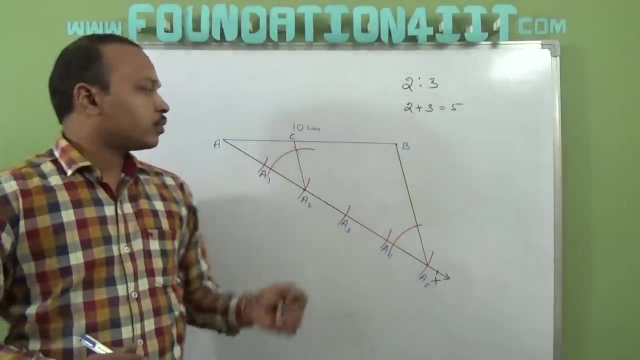 Using scale. you can join it Now A2 to that point Both you join. Yes Does nothing but this line and this line. both are parallel. Now take some C, So AC and CB is exactly 2 is to 3 ratio. 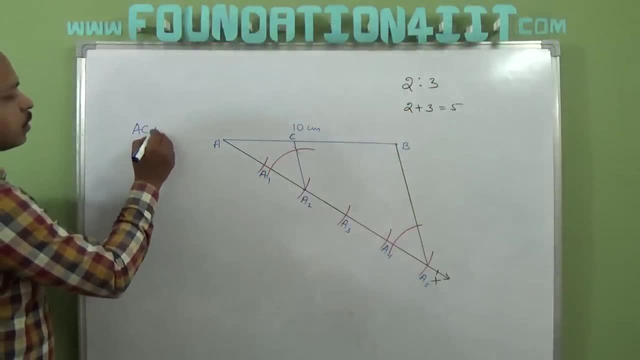 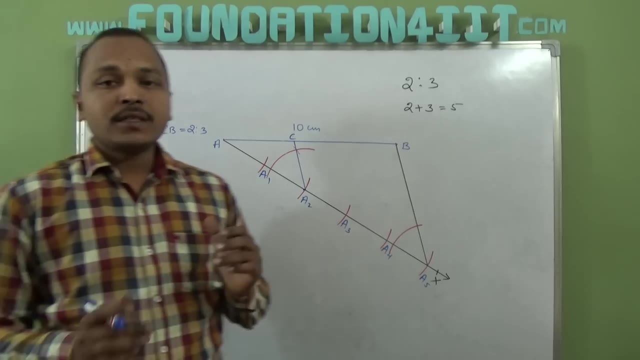 That means AC by. You can see here AC is to CB, AC is to CB, Is equals to 2, is to 3.. Because 3 parts and 2 parts. So here basic proportionality theorem, only The main source for this. 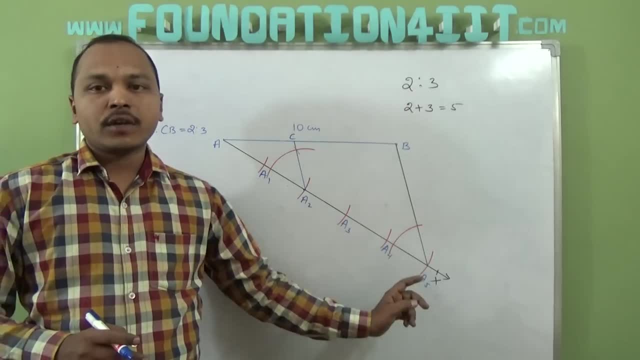 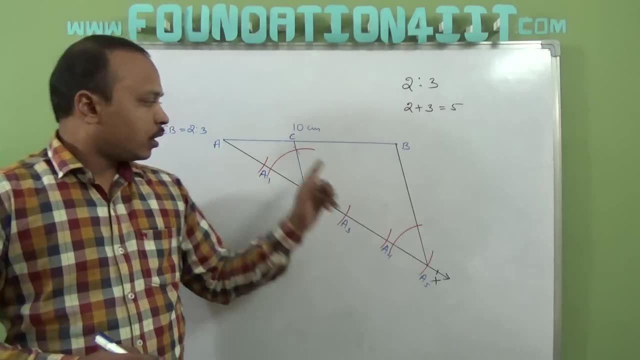 Basic proportionality theorem says: If a line is parallel to any one of the side in a triangle, AB A5 is a triangle right. AB A5 is a triangle Now one. This line is parallel to one of the side, Then that side. 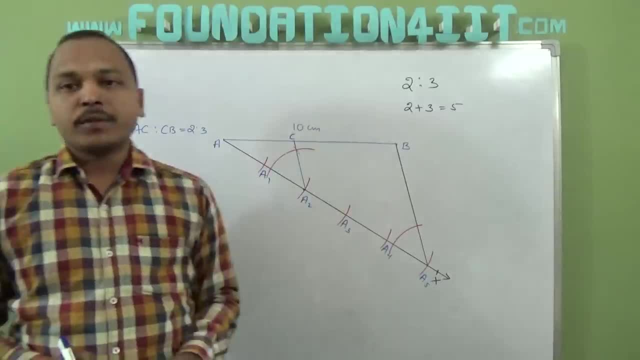 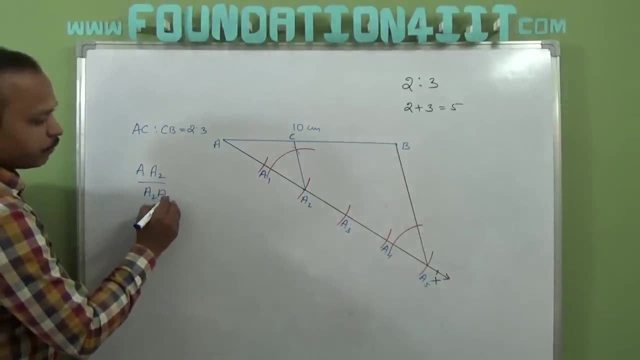 That, whatever that parallel line is there, It divides other 2 sides in same ratio. That means already we know: AA2 by A2, A5 is equals to 2 by 3.. Because this is 2 parts, This is 3 parts. 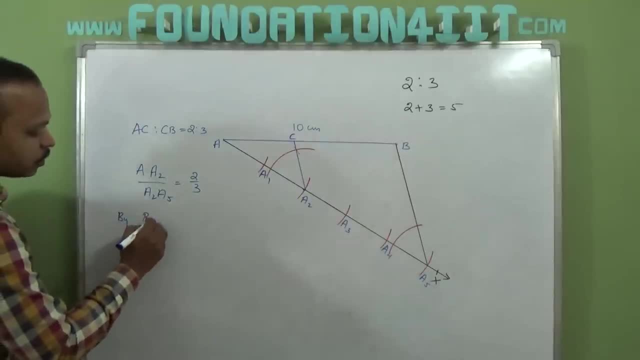 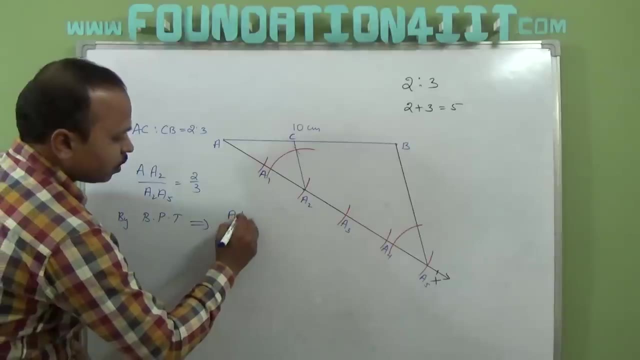 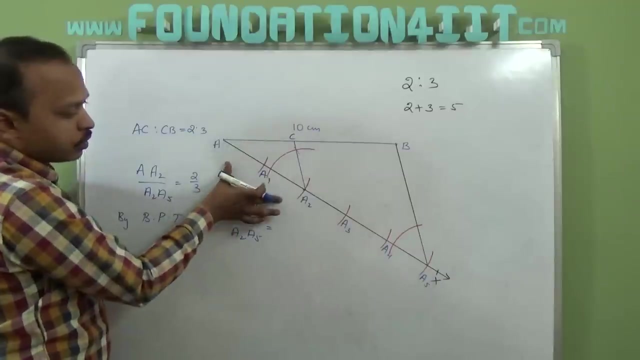 But according to basic proportionality theorem, By using BPT. So basic proportionality theorem: What is AA2 by A2, A5. Means: this line divides other 2 sides in same ratio. So this by this is equal to AC by CB.